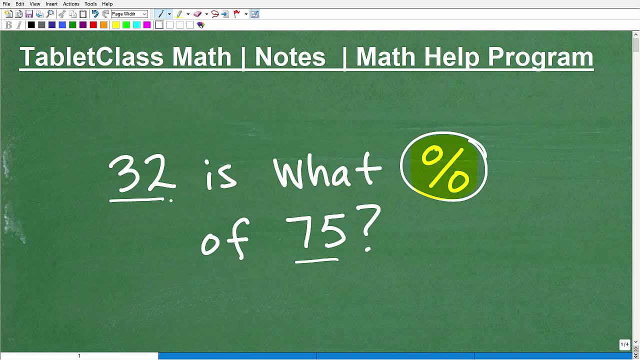 And I would say the majority of people do not know percent as well as they think they do. You know, we do encounter percent almost on a daily basis. If you're at the store, for example, and you see 25% off your favorite coffee machine- let's say it's a curry coffee machine and normally it's $100- and you say, oh, it's 25% off. you know that this cost, this is going to represent $25 off the cost. 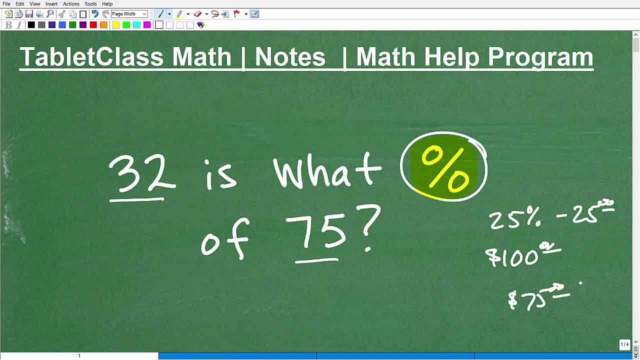 So you're only going to pay $75.. So you know, these are the kind of basic percent problems that we're doing mentally almost all day long. you know, whether it's a credit card, your interest rate, your loan or whatever the case is. 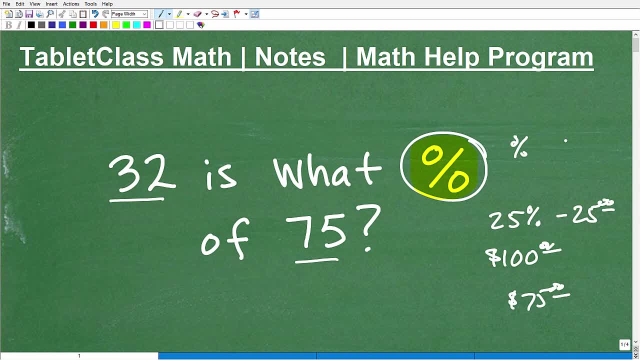 If you have a loan on a car or house. we just see percent constantly. Okay, so most of us have a good feel for it And most of us can kind of mentally do these like sales and discounts and whatnot, And if that's the case, and that's good. 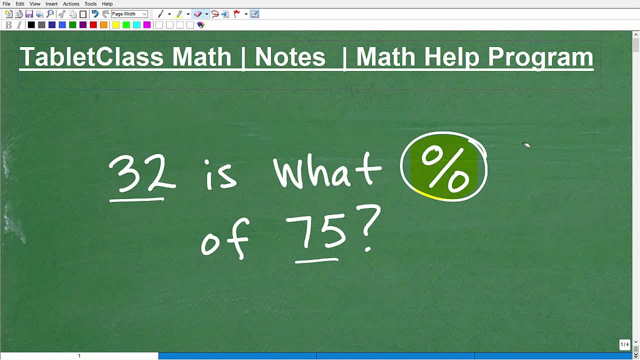 I mean, if you do that, obviously you know that's excellent because that means you're not going to be, you know, missing out on any great deals. But we want to make sure that you can do the little more interesting problems with percent and really master this concept completely. 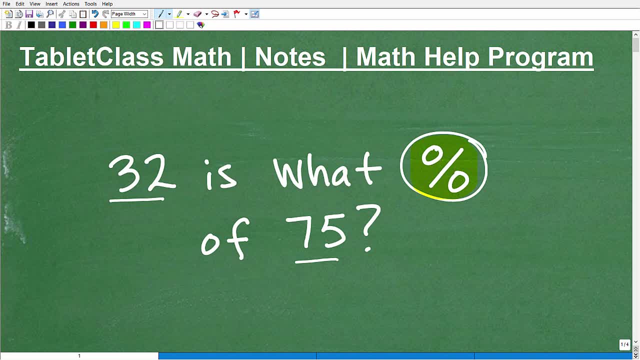 Now, if I gave this question to, let's say, 10,000 people as a quiz, I could tell you right now I'd have all kinds of answers, because a lot of people would be like, oh yeah, percent, Hmm. 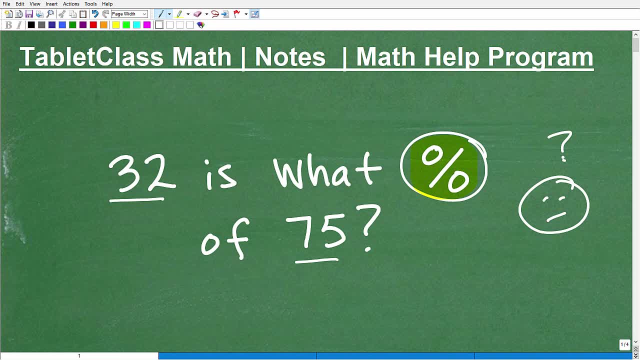 I kind of remember this for like 20 years ago- how to do a problem like this. I think you'd take 0.32 and you multiply it by 75. I'm going to get a lot of that, Or maybe 0.75 times 32, or 32 and divided by 75, or 0.75 divided by 32.. Or you kind of get the picture right. You got to do something with 32 and 75 in order to get the right answer here. But what do we do? 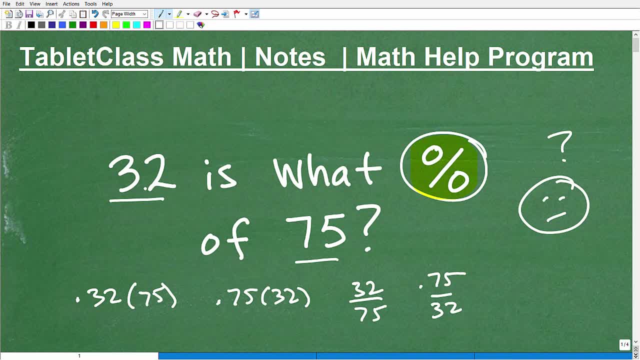 Well, we don't. We don't want to guess, We want to make sure we absolutely know exactly what to do, And we're going to tackle this problem in just one second. But first let me go ahead and quickly introduce myself. My name is John. I'm the founder of Tablet Class Math. I'm also a middle and high school math teacher And over many years I've constructed what I like to believe is one of the best online math help programs there is. I'll let you be the judge of that. if you're interested, You can find a link to my math help program in the description of this video. But if you need to take a full, complete online math course, I offer some. 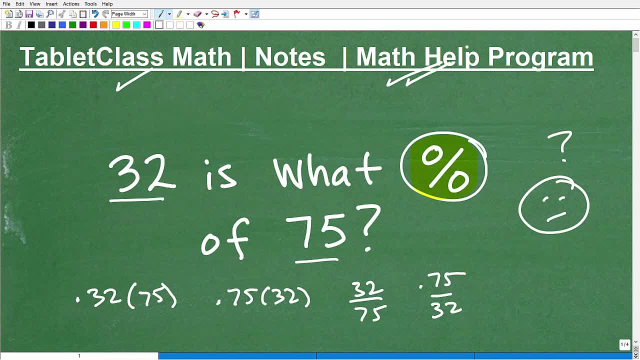 Several, And if you're taking a math course right now and you need help in your course, then you definitely want to check out my math help program. I have complete, comprehensive lessons and I teach you how to solve the most common problems that you're going to encounter in middle school, high school and basic college level mathematics. Okay. so it's taken me years to develop. It's definitely worth your while, if you're struggling in math, to check this out Now. if you are struggling in math or you're struggling in math, you're going to need to take a full, complete online math course. I'll let you be the judge of that. if you're interested, You can find a link to my math help program in the description of this video. But if you're taking a full, complete online math course, I offer some. 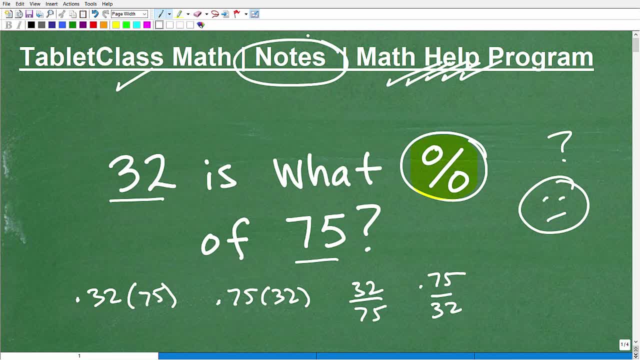 If you're studying math, you need to know this golden rule about note taking. Okay, over decades of teaching mathematics, I can tell you right now it is critical that you take outstanding notes. It's just a rule that I've seen. Okay, those students who have great math notes almost always have great math grades, And the reverse is true. Those students who don't think it's important to take math notes and it's more important to talk to their friends or look at their cell phone or play Sudoku or whatever. 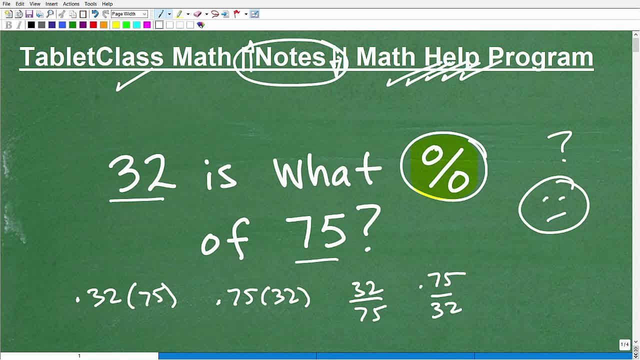 The case is, you kind of get the drift right, That's it. That was me way back in the good old days. I wasn't focused, I definitely wasn't taking good math notes and I paid the price, and you will too. You got to take great notes. So if you're frustrated with your math progress or your math grade, look at your notes and just start approving. But in the meantime you need something to study from. So I actually offer detailed, comprehensive math notes. Those would include pre-algebra, algebra one, geometry, algebra two and trigonometry. You can find the link. 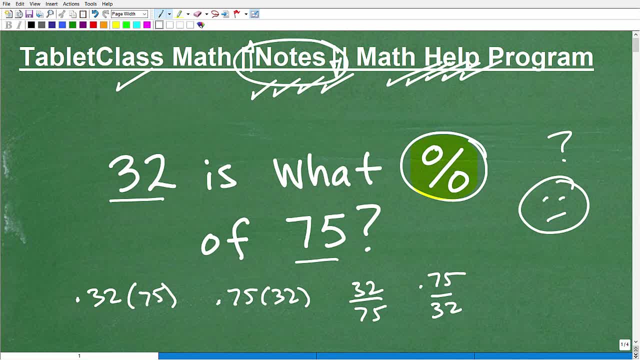 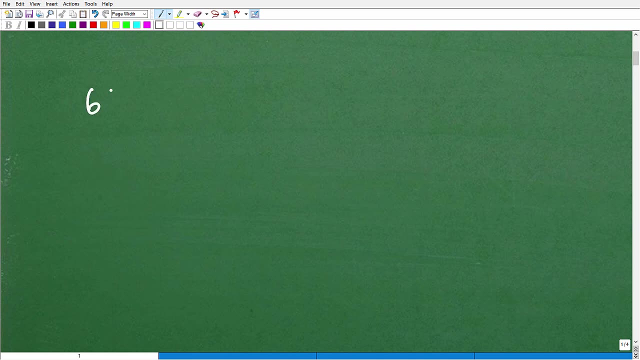 Links to those in the description of this video as well. if you're interested, All right, so let's get to this problem. We don't want any of this. We want nice, happy faces. We want to be a percent master, So let's get to it. Okay, so let's just do a quick review. So if I'm going to say 6% of, let's say, 40. Okay, if I want to answer that question, what do you do, Right? So this is like a basic level percent problem. Okay. 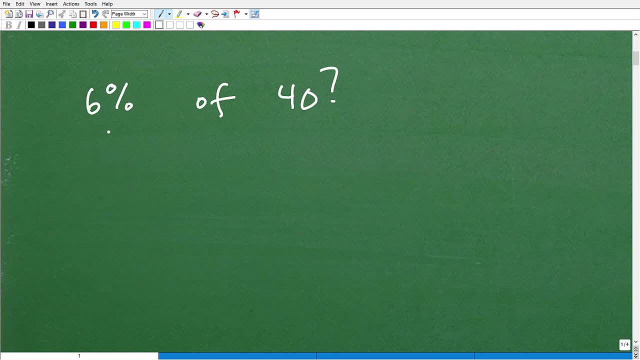 Well, hopefully most of you are saying: oh yeah, don't you have to change this to a decimal and then multiply by this number. Yes, Okay, this is what we need to do And, by the way, I have a lot of other videos on percent in my pre-algebra playlist on my channel. Okay, so this is just. you know. I'm not going to go into every single aspect of percent. I'm going to do a quick review, But if you need to review this more extensively, check out my other videos and my pre-algebra playlist. 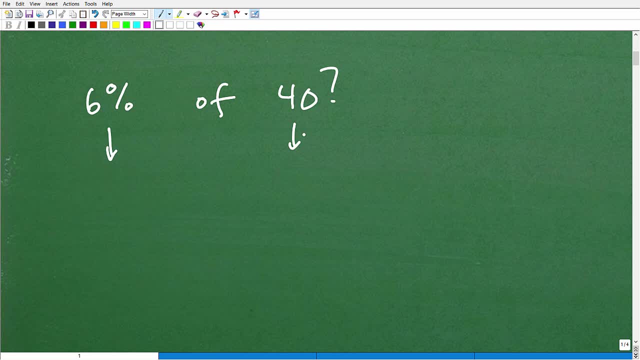 Or, if you really want to get into percent, maybe check out my pre-algebra or algebra one course. Okay, so the way we handle a problem like this is we need to take our percent. okay, like 6% changes into a decimal, And the way we can do that, all right, let's say, do it over here: 6% as a decimal, we divide six by 100.. Okay, So when we do that, 6% is the same thing as 6.5.. 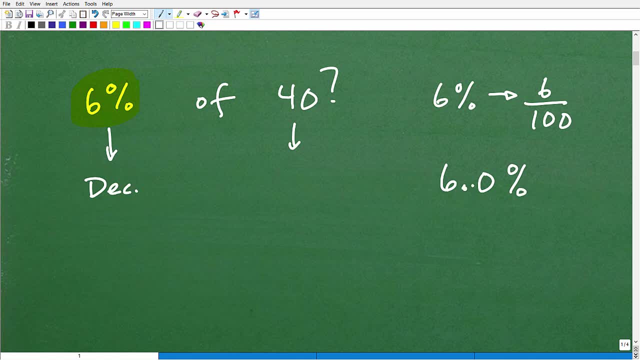 Let's say 6%, Let's say 6.0%, and now I'm saying 6.0% because I want to make sure you understand where the decimal point's at, So what we can do instead of dividing by 100,. 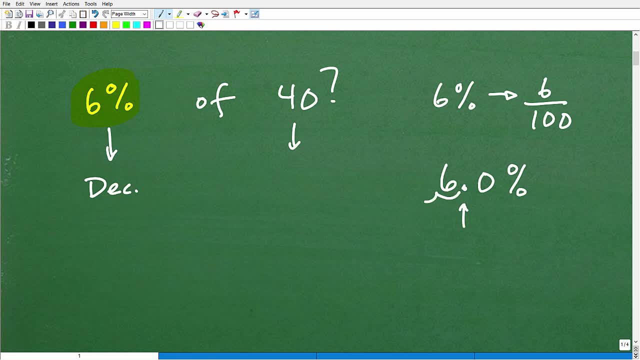 you're going to be doing the same thing if we scoot the decimal point two places to the left. So that's going to be 0.06.. That's the same thing as divided by 100. So you don't have to divide by 100. 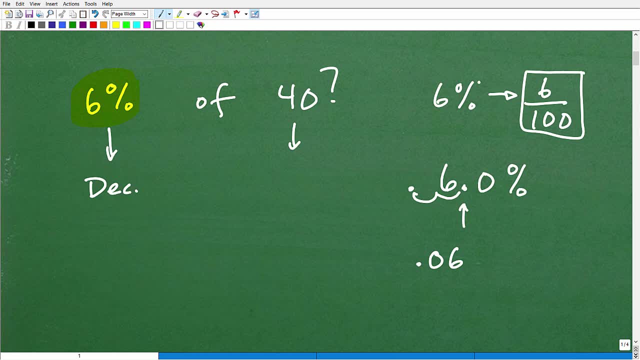 You can just move the decimal point over two places to the left, And that's how we take a percentage and write it as a decimal. okay, so six percent as a decimal is point zero six, point zero six. and then we just multiply that by 40 and we would get our answer. okay, now i don't have a calculator. 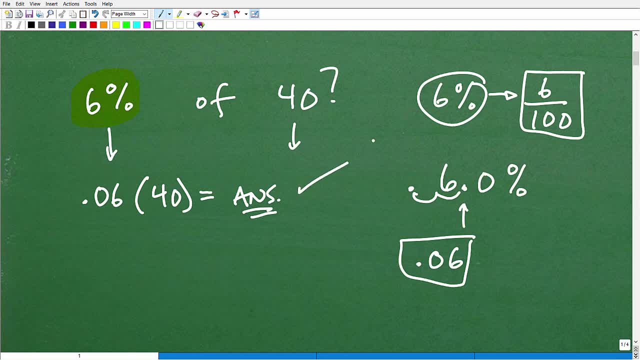 right in front of me. maybe i should, but you could do that calculation and that's how you get the answer. but just this, this is just an illustration of a basic direct uh percent problem. okay, again, we take the percent, write it as a decimal and then we kind of go from there. all right. now let's take 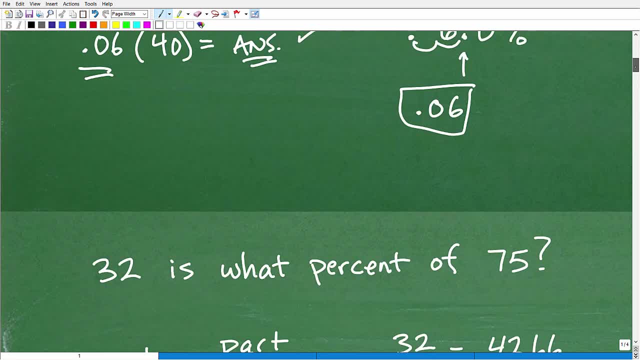 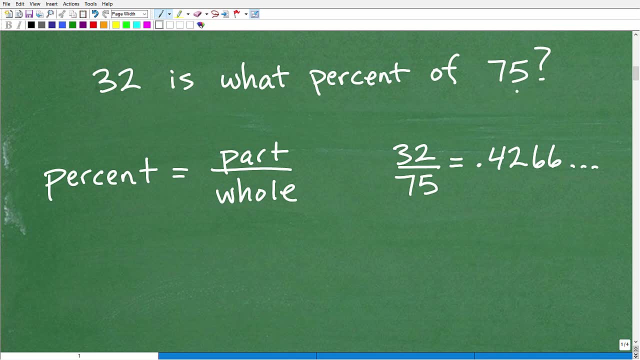 a look at our question and it's just a quick review right on basic percent. so here our question is: 32 is what percent of 75? okay, i don't see any percent signs. the question is in fact looking for the actual percent. so how do we handle this? well, it's a good idea to actually understand. 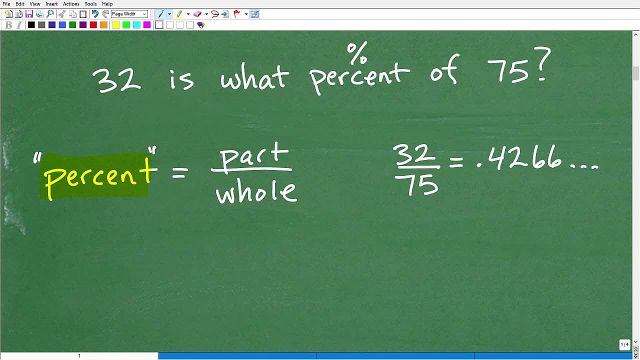 uh, the definition of percent. okay, so percent is a little bit more technical definition of it, but let's just think about it, right. what does percent kind of conceptually represent in our brains? well, it's like a part out of a whole, it's a fraction, right, if i'm saying, uh, 25 is um 25 out of 100. okay, is what's what? percent is 25? 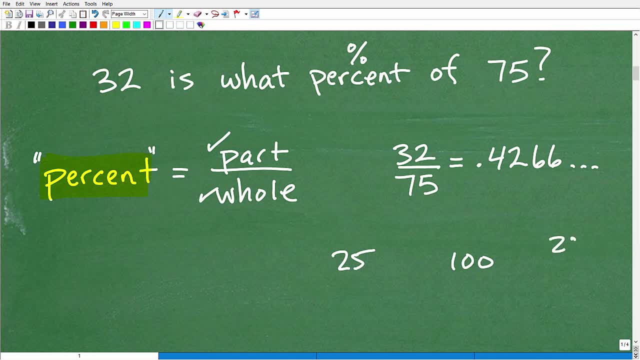 out of 100. well, you're, you might say that's 25 percent. okay, you would be correct, because 25 is the part and 100 is the whole. okay, so we want to be thinking in terms of what is the whole and what is the part. so we look at, uh, this question: 32 is what percent of 75? what is the whole? and 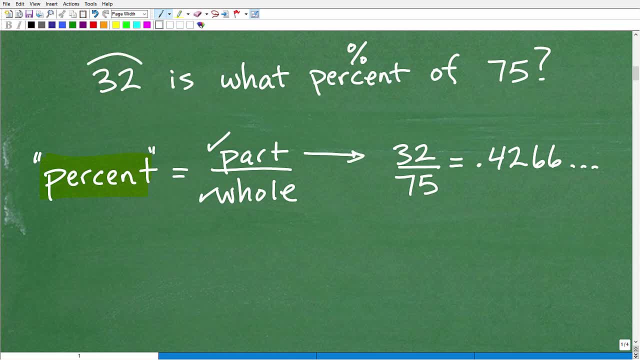 what is the part? well, hopefully you're like. well, the smaller number here, 32, is the part and the larger number here, 75, is the whole. okay, so we want to set this up as a part out of a whole. so if we want to do this, the absolute part of 75 is 0.42666666. this is how we want to write this as a 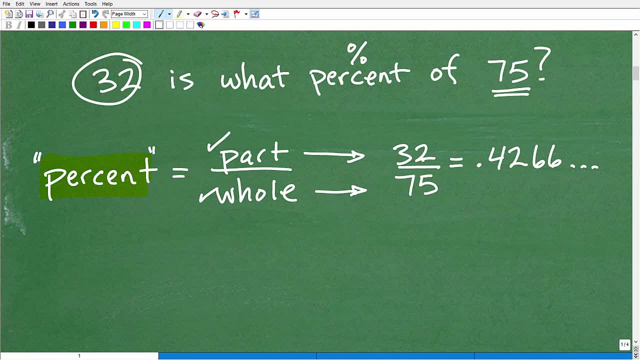 fraction 32 over 75. okay, 32 is the part and 75 is the whole. and now when we take 32 and we divide it by 75, we get a decimal. all right, we get 0.42666666. just keeps going on, and on and on. 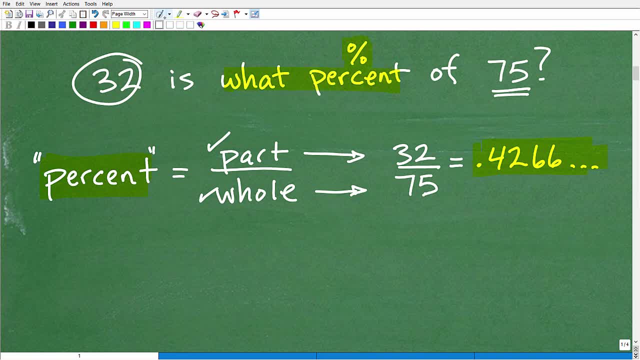 now a question is asking: what percent? okay, so some of you might just do this math and this, do this calculation, and stop right here and give me this as an answer. all right, what's the matter with this answer? well, this answer: this is a decimal, okay, this is not a percent. okay, we'd like to. 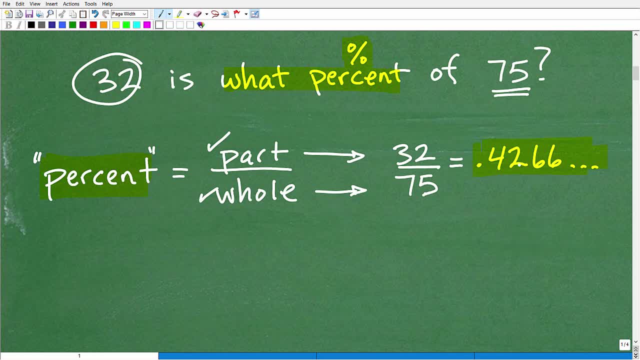 see things as a percent. so how can I write this point for two? let's do it down here: actually point four, two, six, six and so forth. how can I write this as a percent? well, if you recall, when I had six percent, that was like six point oh. 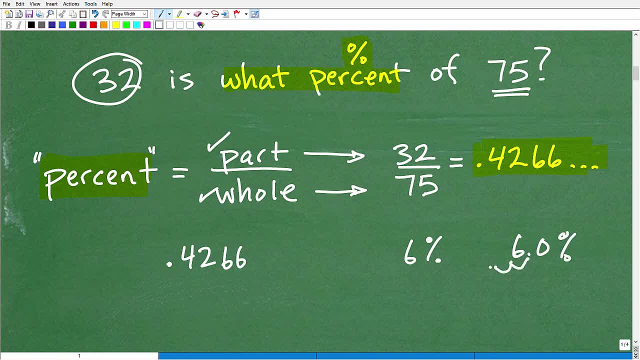 percent. to change this into a decimal, I move the decimal point two places over to the left. okay. well, when you are given a decimal like point zero, six, and I want to express that as a percent- you move the decimal point the other way- okay, back to the right, and then go get back to your six percent. so same thing here. 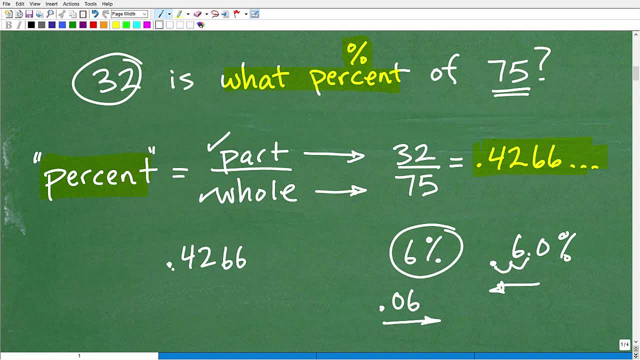 point four, two, six, six as a decimal. okay, this is a decimal. I want to see this as a percent. I just have to move the decimal point two places to the right now. okay, which is the same thing as multiplying by 100. so I think me one and two, so that. 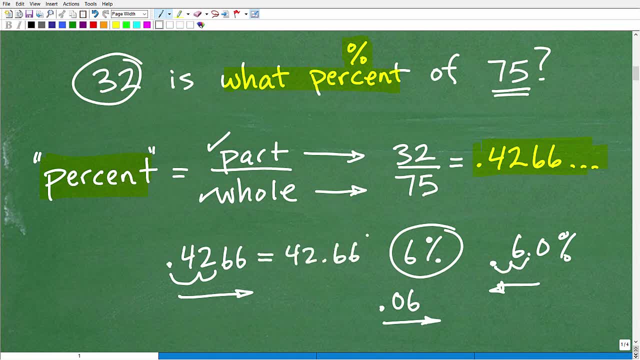 would be forty two point six, six percent. forty two point six, six percent is the answer. now let's just take a look at this right. thirty two is what percent of seventy five? well, I'm saying it's forty two point six percent. is that logically, you know? does this make sense to you? like you always. 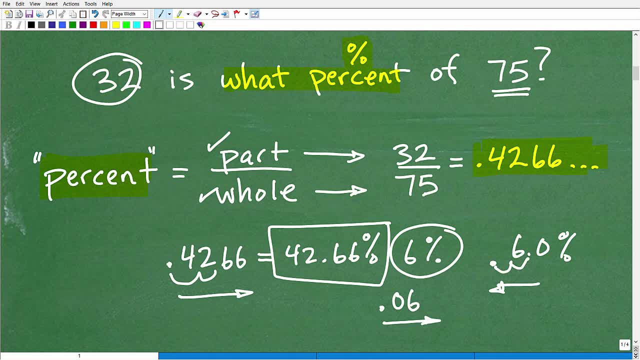 got to think about your answers and just give it kind of the smell. test the reality, test, right. so 32 out of 75. if you just kind of initially think about this, double this number for a second, that's 64, right? so 32 out of 64, that's a. 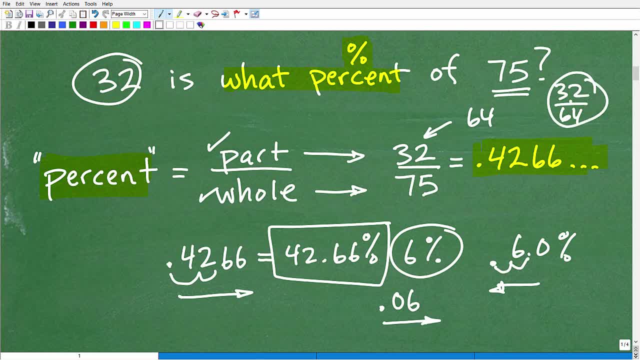 fraction that's equivalent to 1 half or 50 percent. so this denominator 75 is bigger than 64. So this is not going to be quite 50%, but 42.66% seems reasonable. okay, And you always should look at your answers and you know kind of think about them. 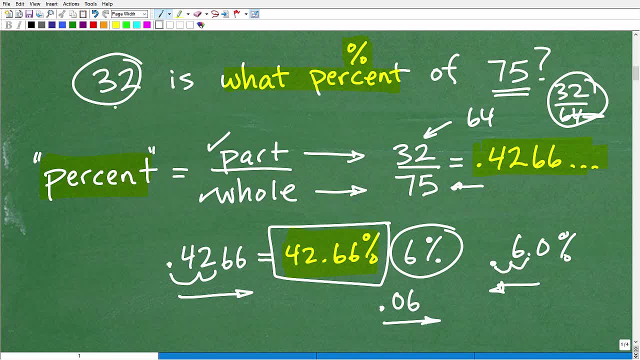 Is the answer reasonable? Because I could tell you right now: 32 is what percent of 75?? I would have students give me like oh, it's 3%. I'm like, yeah, does that even make sense? Okay, think about your answer. 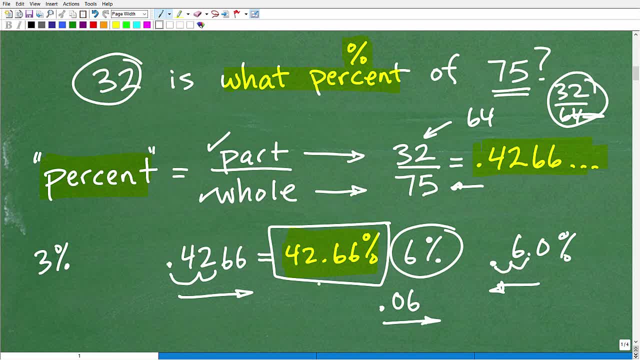 Think about you know the value of the answer and match it up to the question and then ask yourself, oh yeah, no, this does it does seem realistic. okay, Always try to do that. Sometimes you can't do that in every single question, but with percent, the more you practice it, the better feel you're going to get, for you know, kind of reality checking your answers. 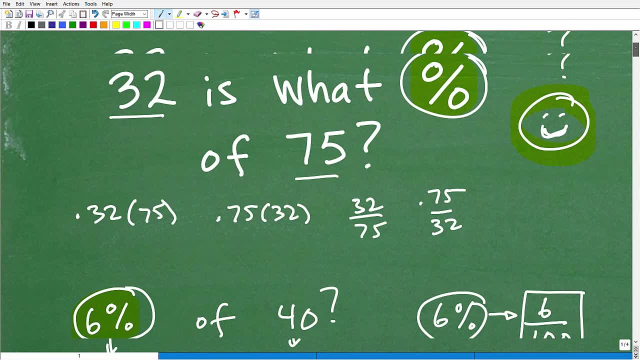 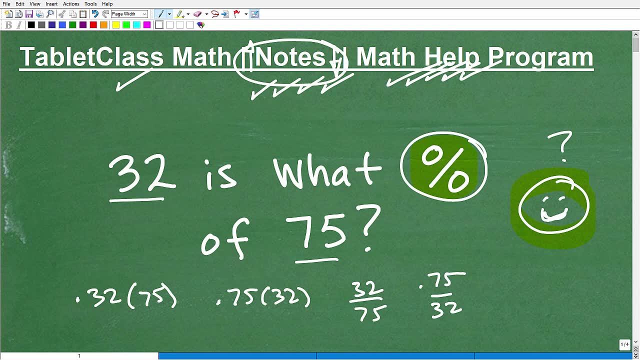 Okay, so there's other types of percent problems that you can do, for sure, But anyways, you know, I think the thing is Is percent is more than just the basic stuff and we just don't want to be guessing. okay, You know, when you got to figure something out, you got to figure. you know, you got to have absolute certainty in this. 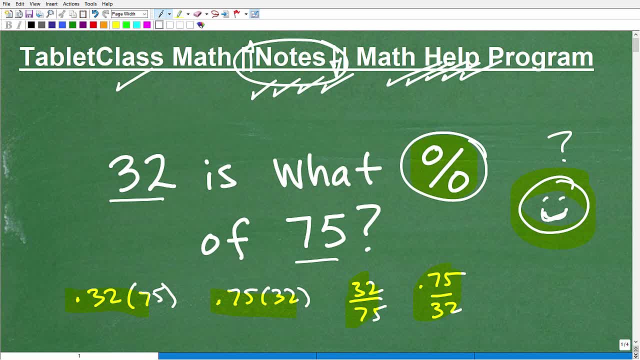 Now, if you were able to do this and it was like a piece of cake and you were like, yeah, I got this as with no sweat, then give yourself an A+, 100% and maybe a few stars as well, okay. 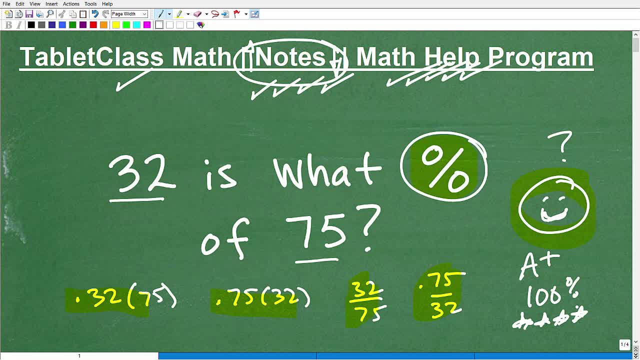 Because you definitely deserved it. You know your percent and that's good stuff. Now, of course, I could give you more challenging percent, I promise, and actually have a few more interesting problems. Again, check out my pre-algebra playlist. you know, I think you'll I've definitely put more of my basic stuff there, but if you like this video in some way, please consider smashing a like button 100%. that would definitely help me out big time. 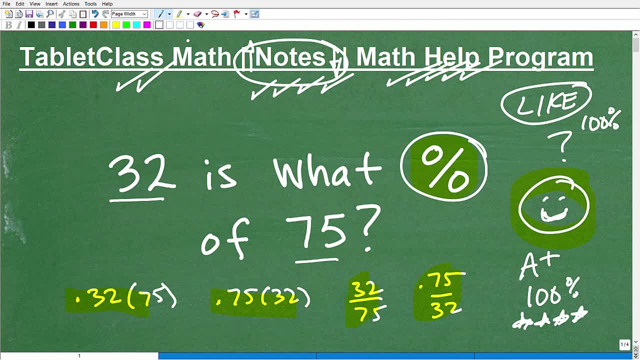 And if you're new to my YouTube channel, please consider subscribing. been on YouTube for a long time, Love teaching math, love the platform. I think I've been over YouTube for over 10 years at this point and I have hundreds and hundreds of videos organized in various playlists: basic to advanced math. 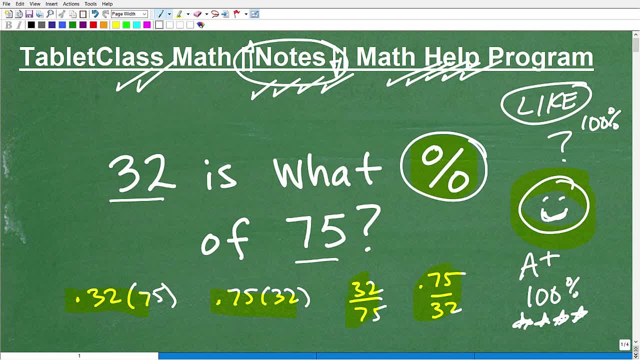 So if you like my teaching style, there's a ton of help there. but if you really want my best help, check out the resources by following those links in the description of this video. But with that being said, I definitely wish you all the best in your mathematics adventures. Thank you for your time and have a great day.